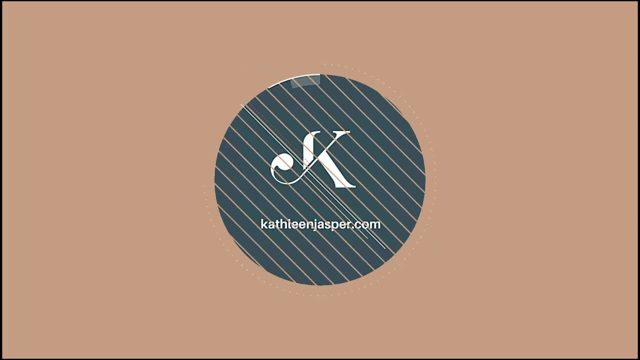 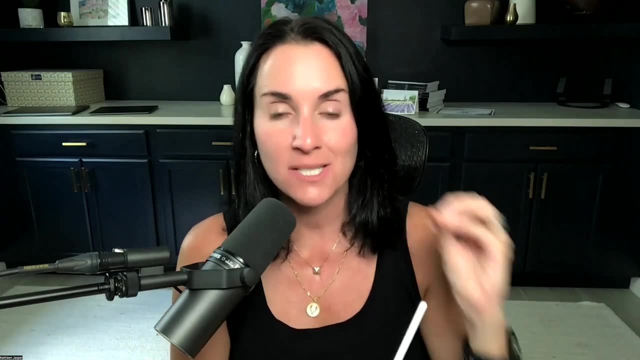 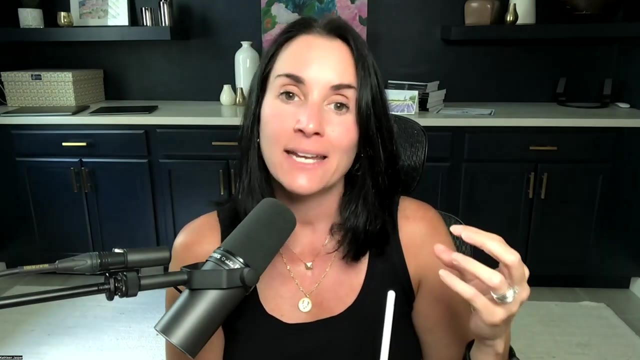 Let's get started. All right, I want to start this video off with a huge disclaimer. What I'm going to show you today is not released by ETS. This is not an exact science, and I'm going to show you how to calculate your raw score into your scale score, but it is by no means an 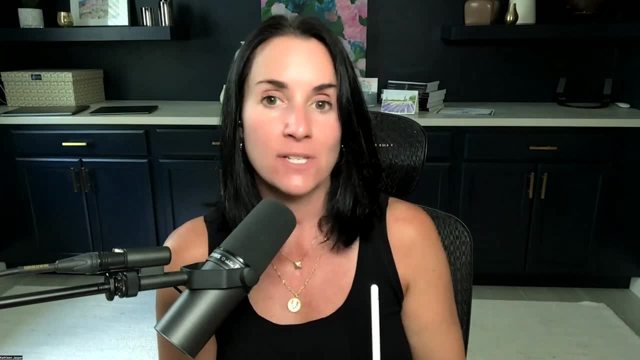 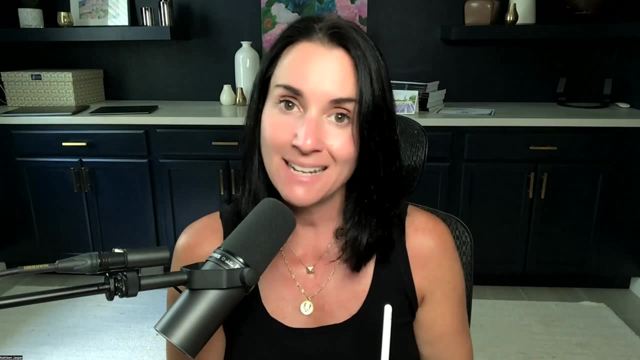 exact science. Some of you are really interested in how these exams are scored, and I totally get it. You want to know what's up. You want to know why they're grading you the way they're grading you. so it's totally understandable, but ETS does not release that information. 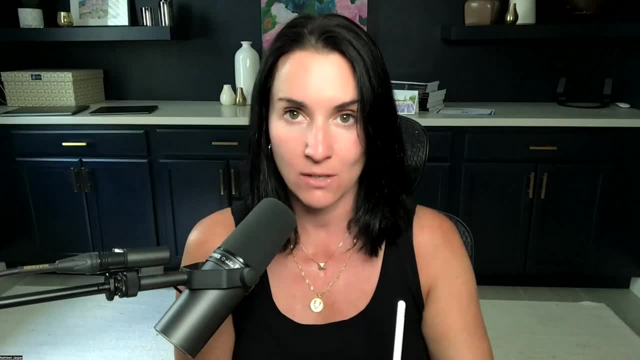 They just talk about the fact that they convert your raw score to a scale score, and I'll talk about that in a second. But the way they do it is: they convert your raw score to a scale score, and I'll talk about that in a second. 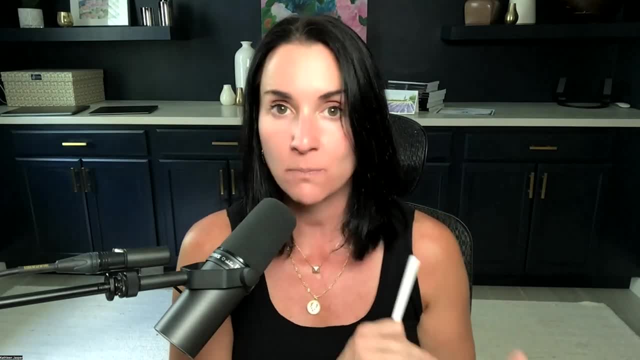 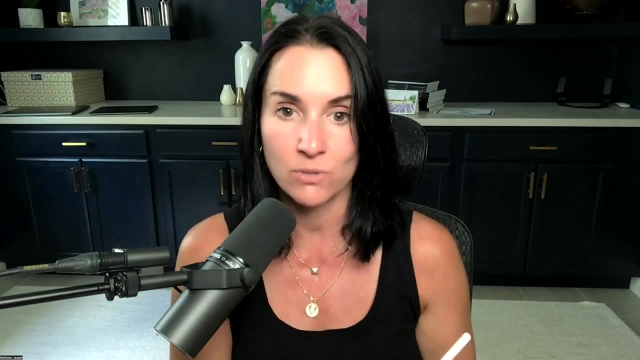 However, I went through a couple of other test prep companies, looked at a ton of information online and looked into some universities who have released this information and I'm sharing it with you today. But again, huge disclaimer: this is not endorsed by ETS. This. 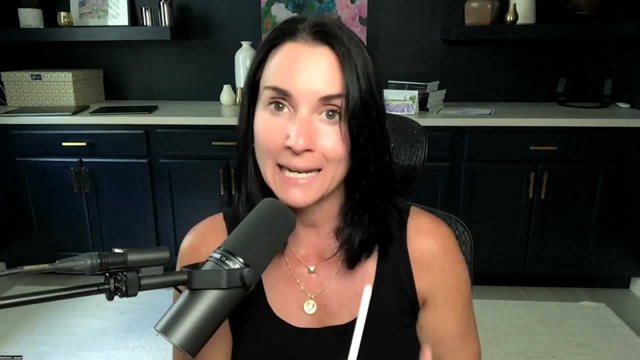 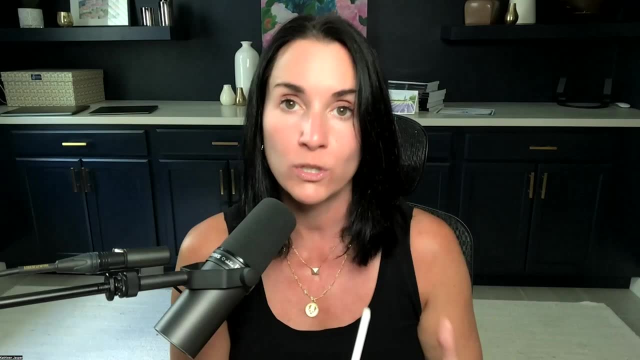 is not an exact science. This is an estimation and a way for you to kind of understand how you take your raw score and turn it into a scale score, but it should not be the only way in which you determine your readiness to take the exam. 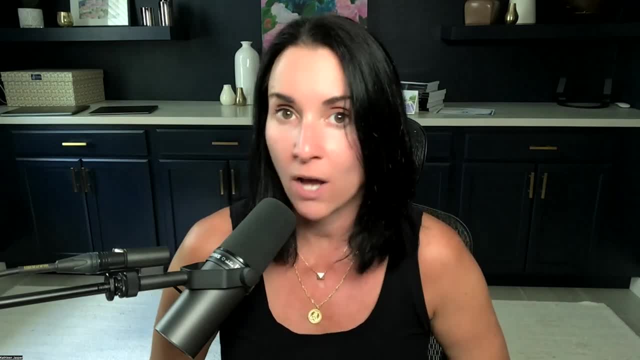 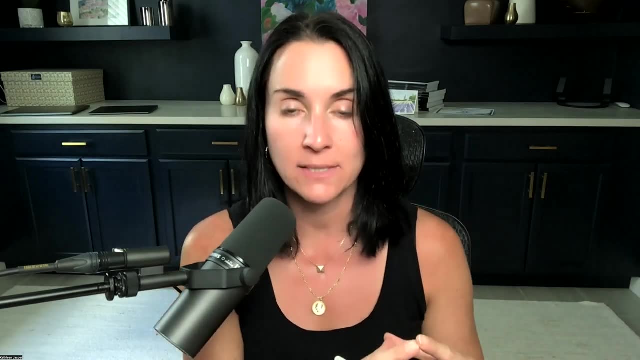 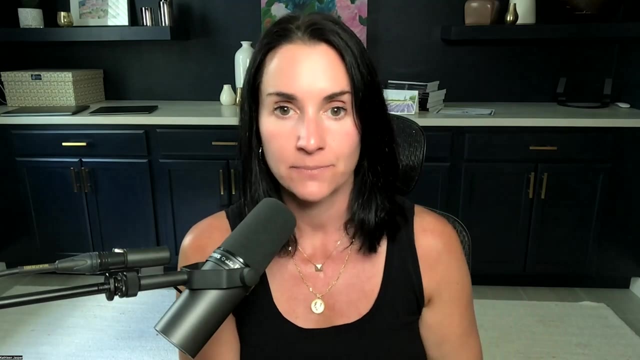 Okay, First let's talk about the difference between a raw score and a scale score. okay, A raw score is the total number you get correct on a test. So let's say you take a test that has 100 questions on it and you got 68 correct. Your raw score is 68.. That's your raw score. 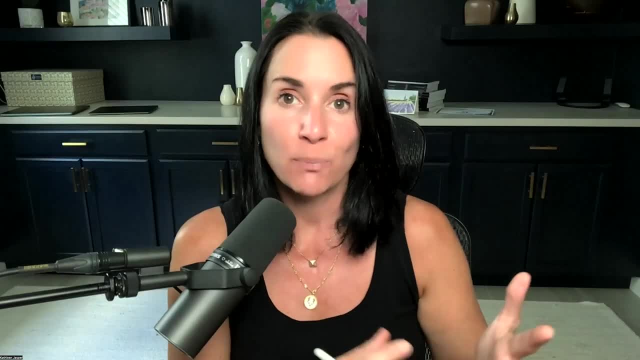 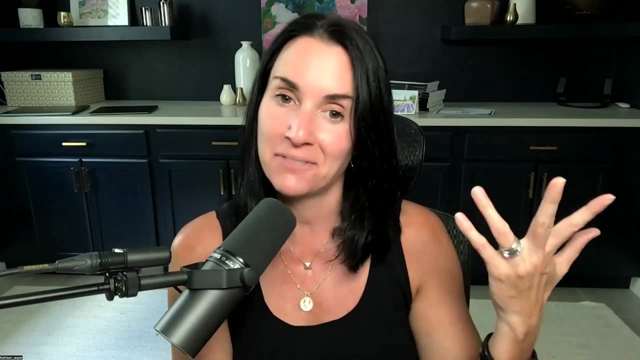 because that's how many you got correct. Now, because the test is out of 100, your percentage correct is also 68. It's easy, because it's out of 100. So let's talk about the difference between a group that has 100 questions and your percentage correct is out of 100. If 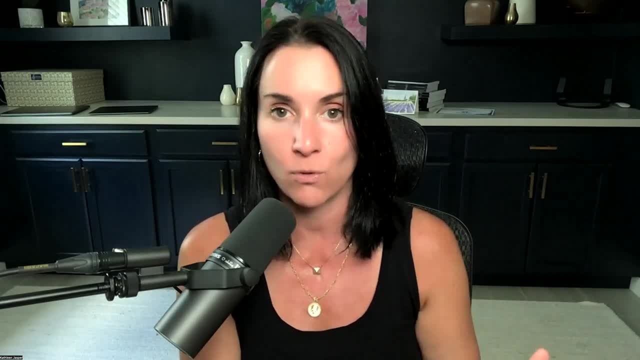 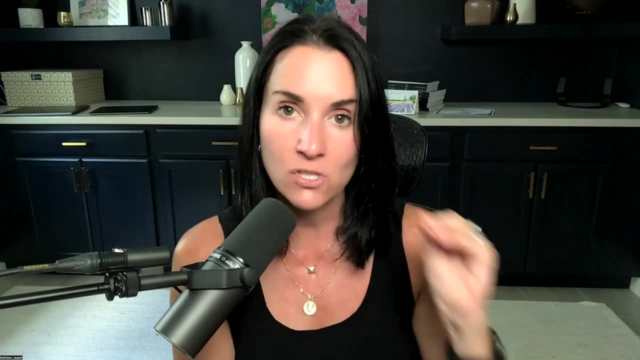 it was out of another number. it would be more difficult for me to calculate off the top of my head, So I'm using 100, alright. So raw score is just a straight up how many you got right out of all the other questions. all right, And in this case it would be 68.. 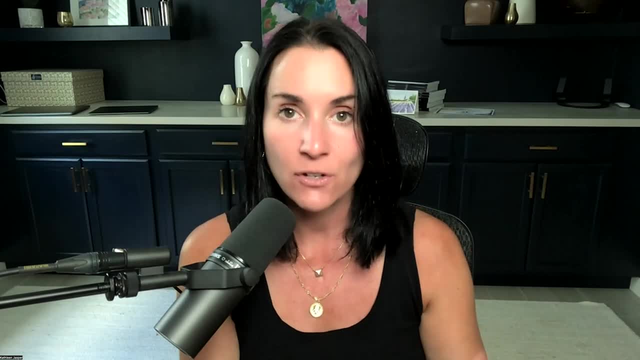 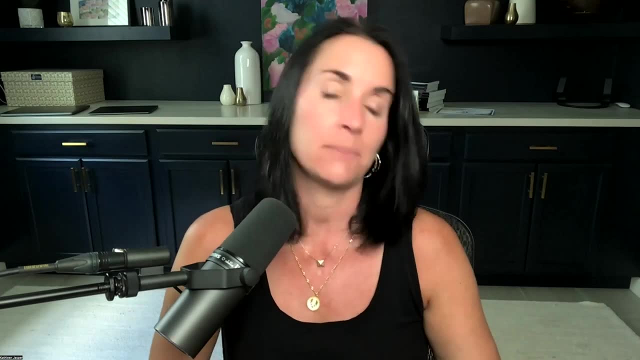 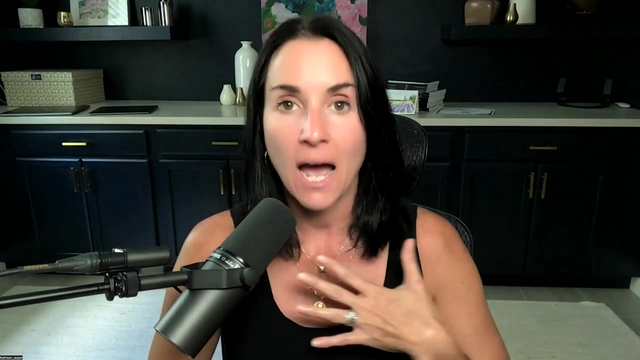 Now a scale score is when the testing company converts that raw score into a scale score to kind of level the playing field among all the forms of the test that are administered. you are going in to take the Praxis teaching reading 5205.. And I am going in to take the 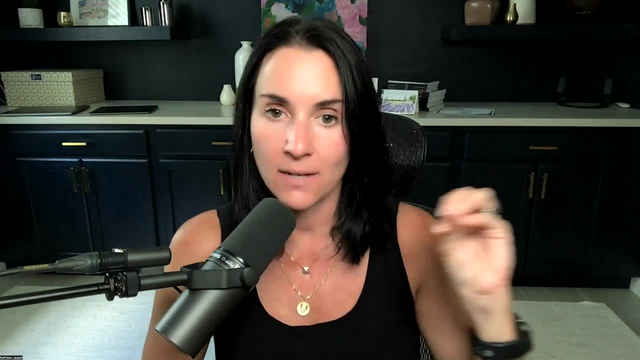 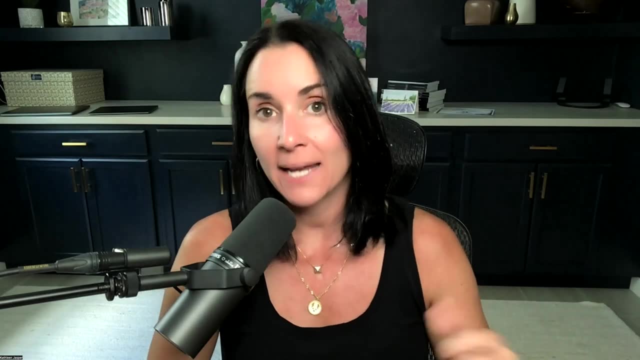 Praxis, reading 5205.. Let's just estimate it has a hundred problems on it. It has more than that, but let's just say, for the sake of this video, it has a hundred questions on it. Okay, And when I go in I get a form of the test, form A, and you go in and you get form B. 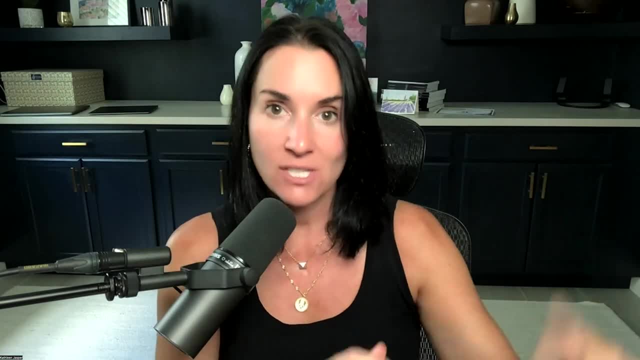 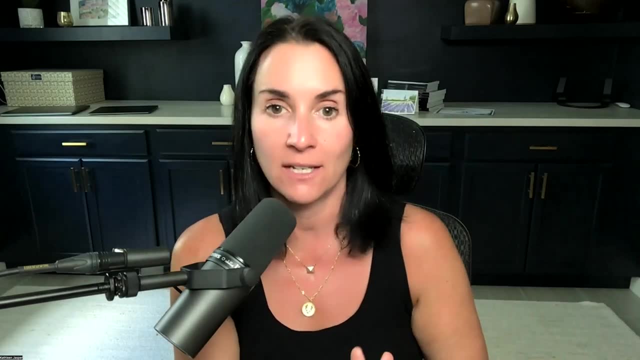 You are going to get a different test than I am, because if they just gave the same test over and over again, the test wouldn't be secure, It would be unreliable, and they call it item fatigue, meaning these items have been seen over and, over and over again. What are we going to do? You are 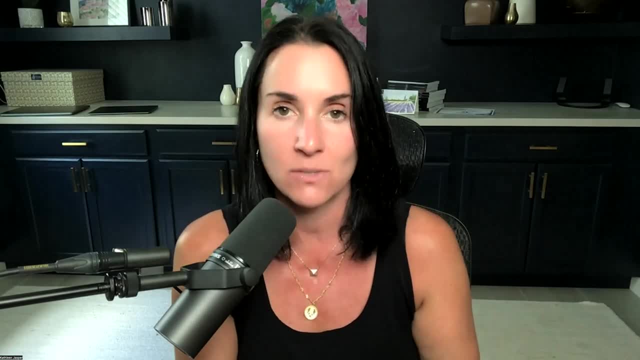 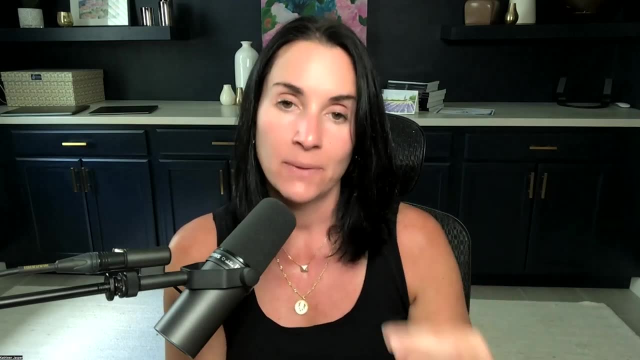 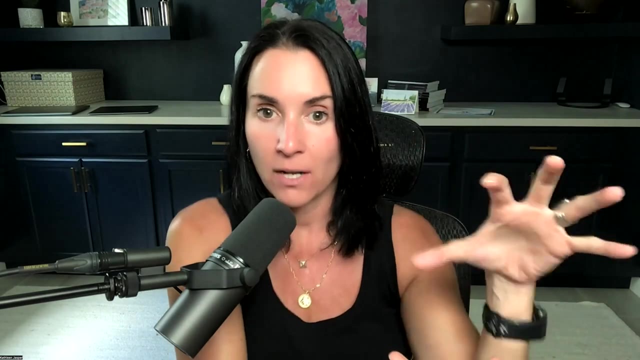 going to share them. You are going to talk online about them. This happens, right. So in order to keep the test secure and reliable, they have different forms of the exam and those forms are populated by item banks, meaning there is an item bank. for phonological awareness, There is an item. 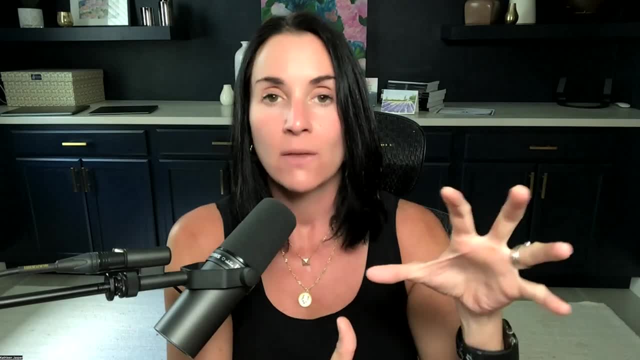 bank for phonological awareness. There is an item bank for phonological awareness. There is an item for phonemic awareness. Remember, we're talking about the teaching reading test. There are item banks for the writing there, you know, and so from those item banks I get 20 problems for. 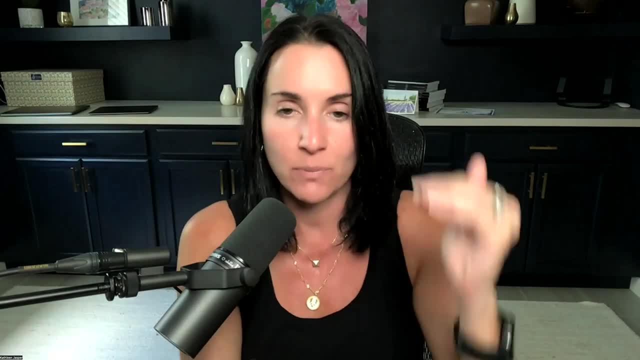 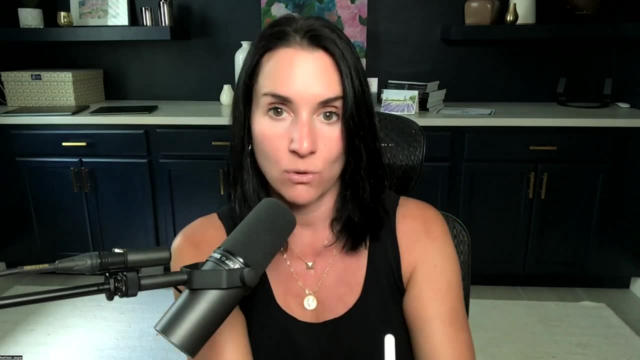 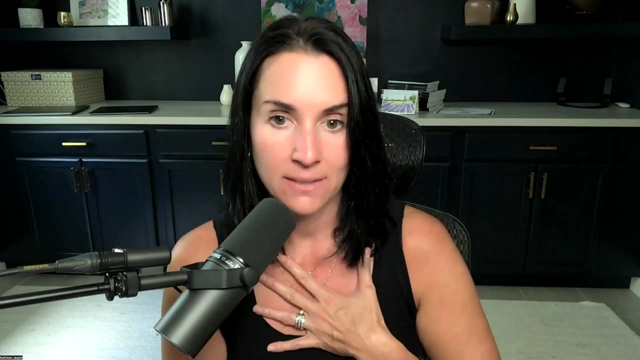 phonemic awareness, I get 30 problems for writing, or whatever the percentages are for the content categories, And so my hundred question test looks different than your hundred question test, right? So let's say we both go in and I get 70% correct And you get 70% correct. You got a 70 and I got a. 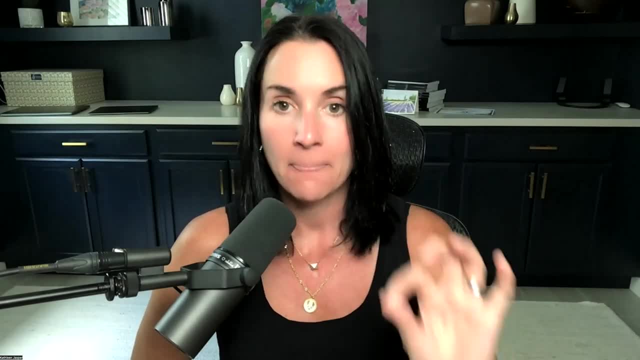 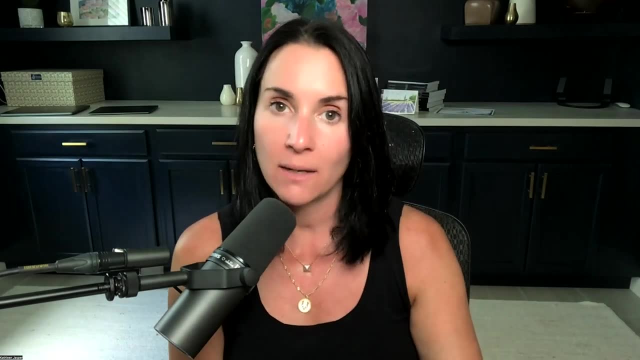 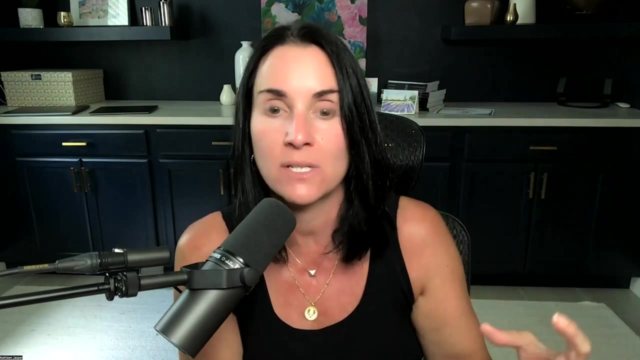 70. Our raw scores are both a 70. But let's say your test had higher complexity items on it, meaning you had more items that had those choose all that apply, or the real heavy scenario, questions with the very long answer, choices that are that have more cognitive demands. 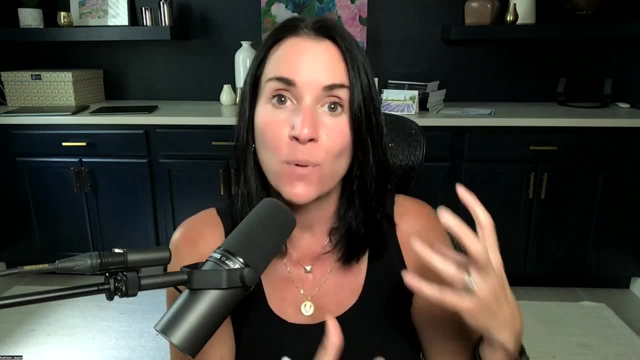 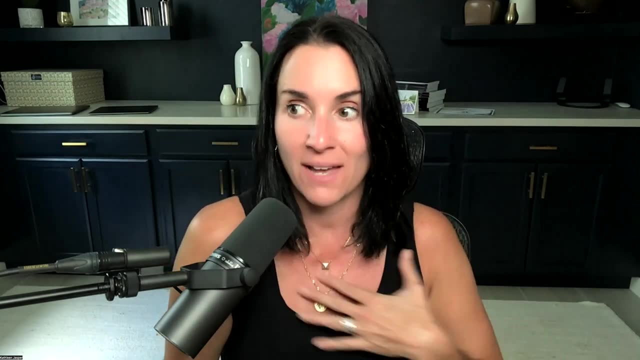 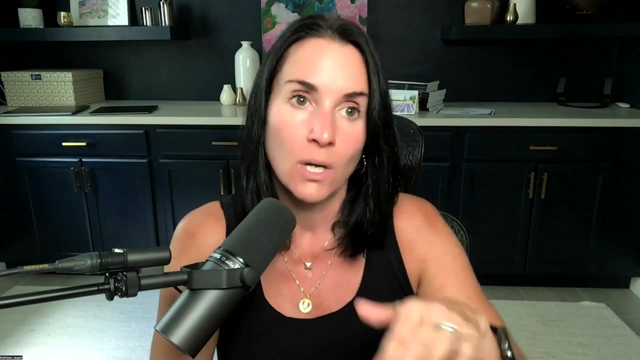 And those questions are worth more points. they're weighted, And so, in order to level that playing field so that my score reflects my score and your score reflects your score, they put a scale score in place in order to even out those differences. So let's say: you only got. 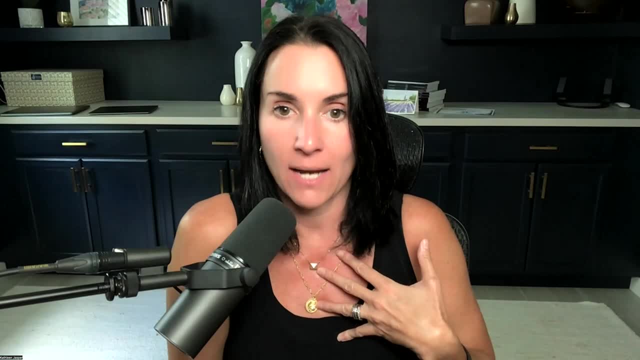 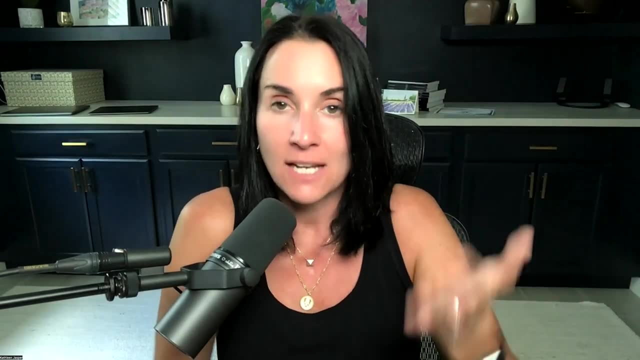 50 correct on your exam and I got 60 correct. But your exam had harder test items on it- your scale- So your scale score is going to go up And it's going to even it out. Yeah, I got 60. Correct, But. 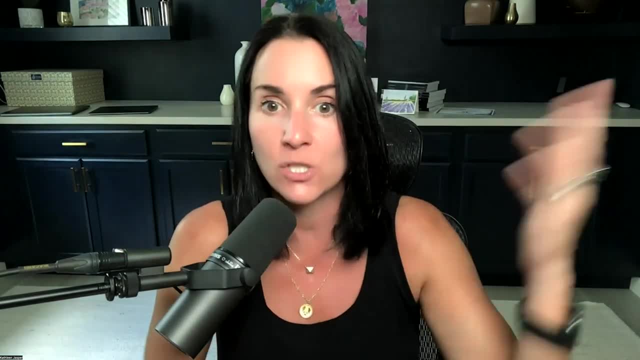 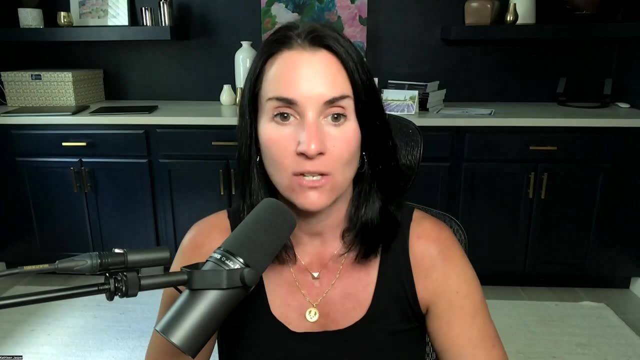 all of mine were easy And you got 50. Correct, And you had 10 that were much harder than mine were noticed that they would have to put in a measure in order to even that out. So that's why they use a scale score, because they have to use different forms of the test, And that's how it. 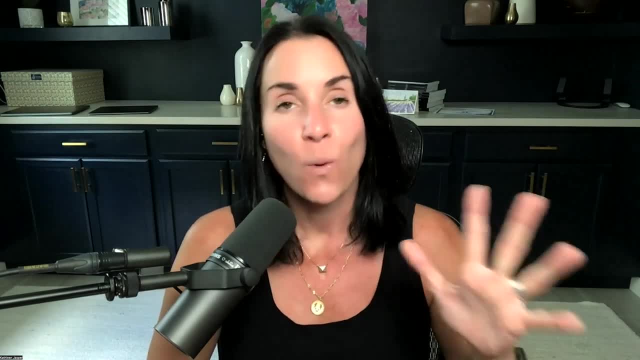 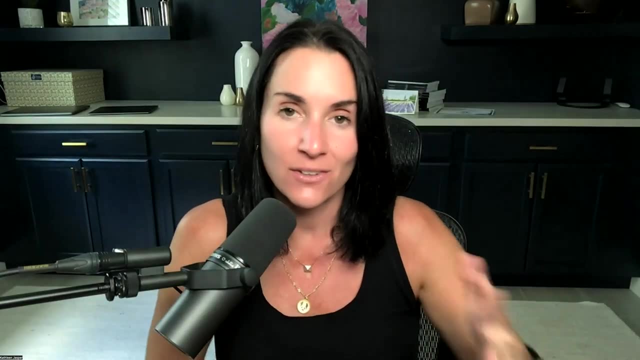 works. Now, How do they figure out your scale score? Well, there's all kinds of mathematical wizardry and trickery. Not really, It's a statistical thing. They do, But I don't know how it's done And ETS does not release it. So what we've done is we've 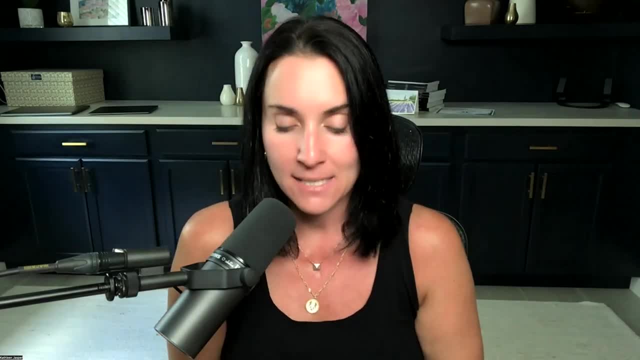 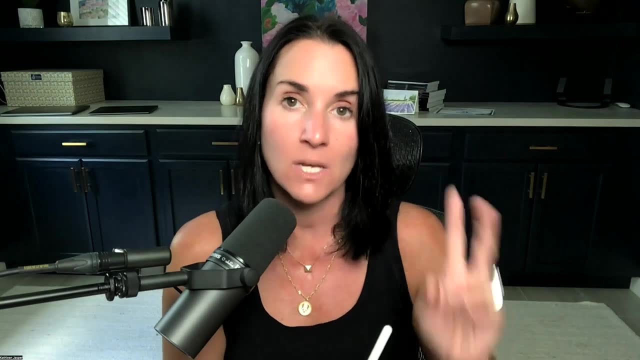 used a little conjecture, use a little research, And I'm going to show you today how you can kind of calculate it All right. So just remember that a scale score- and for the praxis exams it's 100 to 200- is the scale score. So they convert that raw score into a scale score, And that's what. 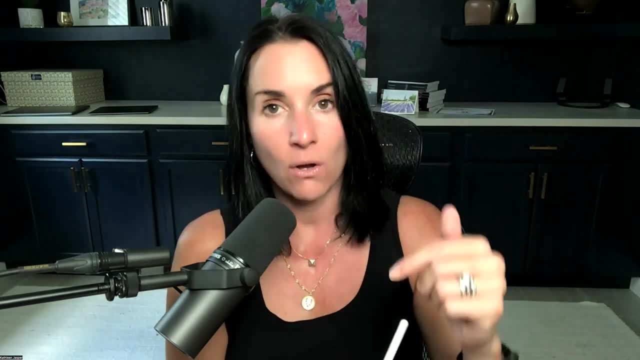 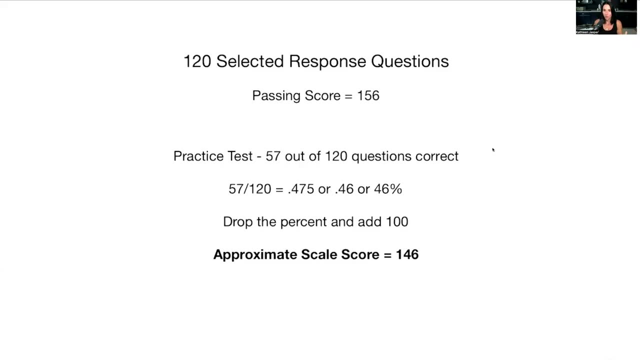 you see when you get your test results on the computer and also on your score reports that come in the email, you know, a few weeks after you take the test. So that's what you see when you get the exam. All right, So how does this work? How can we kind of calculate this? Well, let's just 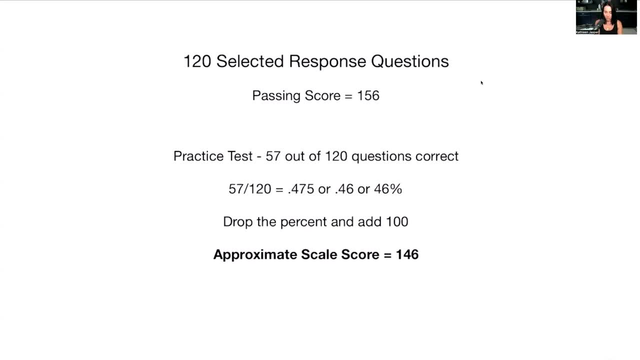 say that we are taking a test with 120 straight up selected response. Okay, there's no constructed response, It's just a multiple choice test. And let's say, in my state for this exam, the passing score is a 156.. All right, Well, if I want to kind of calculate where I am doing the practice. 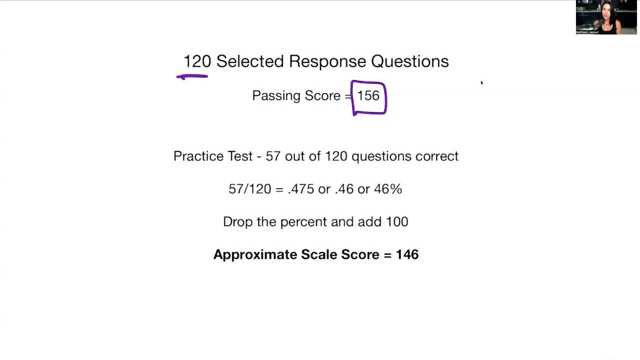 test in the study guide. I could basically just calculate my raw score and do a little formula here. So let's say that the first attempt I have a, I got a 57 out of 120 questions. Let me make sure my math is right here. So 57 divided by 120.. Okay, good, So my raw score is a, is a 57.. 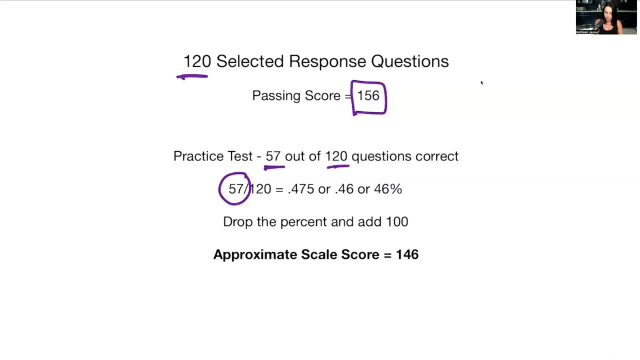 Now my percentage correct is a 46% because I divided 57 by 120.. Just like you would in a classroom, if you want to figure out your percentage on a test, you would take how many you got correct divided by the total and you would get the percentage. 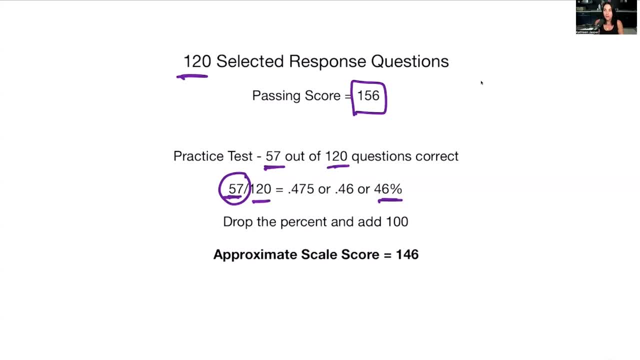 Okay, So in this case I got a 46%. Well, if I wanted to figure out an approximate scale score, and this is with no waiting and no differentiation between hard questions and easier questions. that's why this is an approximation- you could drop this percent at a 100 and you would get a 146. 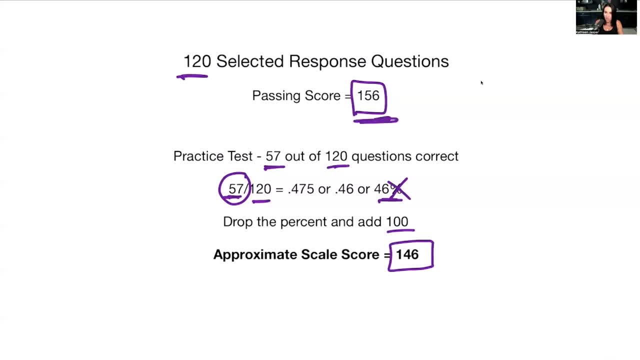 And so we're not there yet, you are not in this range at all And you're not ready to take the exam. Well, let's say that I go in, I study the study guide, I watch the videos and all of that, And I go in and I take a new practice test I take 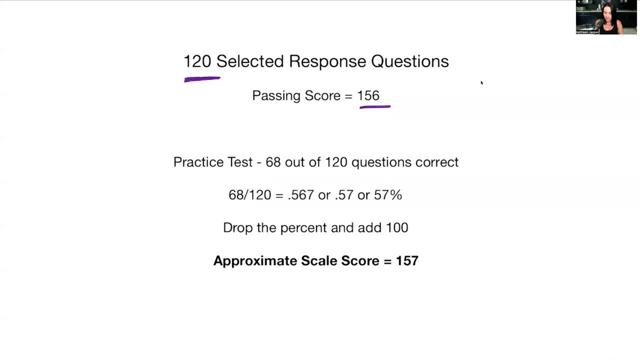 practice test to same thing: 120 questions, And for my state I need a 156.. Well, this time I got 68 out of 120.. Make sure my math is correct on this one as well, And it is, So my raw score is a 68.. 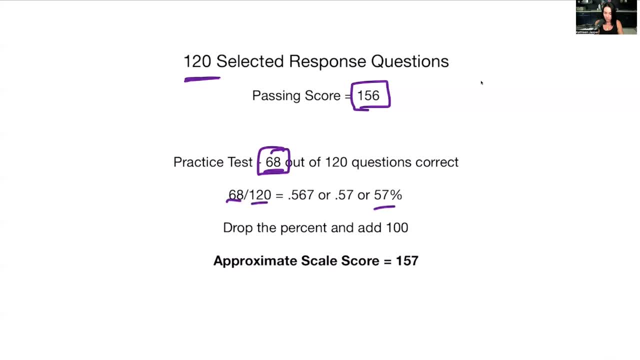 Well, to get my percentage correct, I take 68 divided by 120, I get this 0.567. And I round- you want to round- to the nearest 100th and I get 57%. Well, if I drop the percentage at 100,. 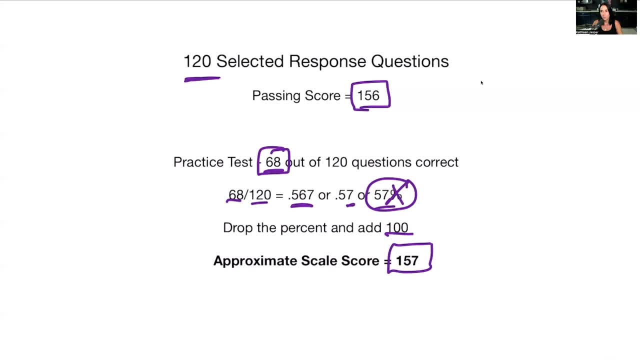 I'm at a 157.. This is why it's problematic to rely solely on this particular measure. Look how close it is. Yeah, I'm in passing range according to this, But I'm still very close. And, let's say, I can't, you know, calculate the weight of the questions, how difficult they are. 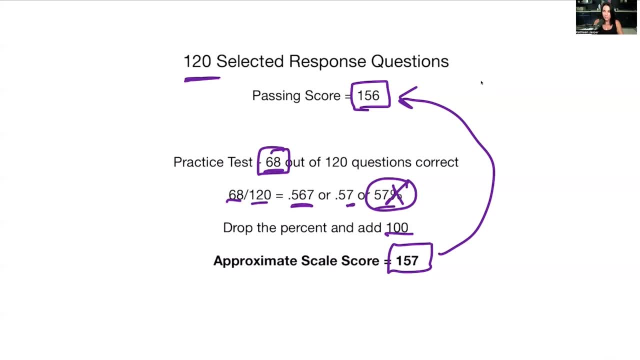 This can be problematic and not an actual measure. So it's okay to use this formula- And you know I like it and all of that- But really you should be shooting for a 75% correct on your practice, on your practice exams, in the selected response, because that puts you in the 100% safe zone. 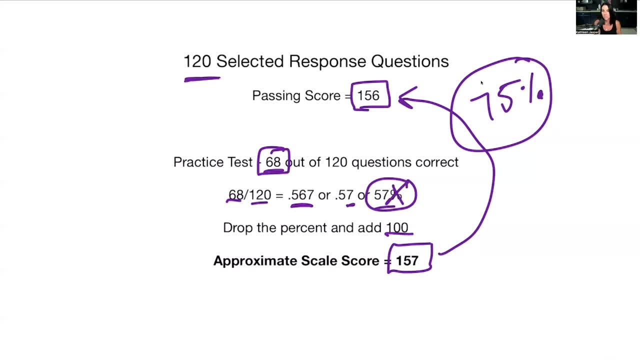 whether they're low complexity, high complexity, mid complexity questions. you know that if you're getting 75% correct, you are in the zone. Now you don't need 75% correct to pass. In many cases you need a low D, a high F, a low C to pass these exams. So just understand. 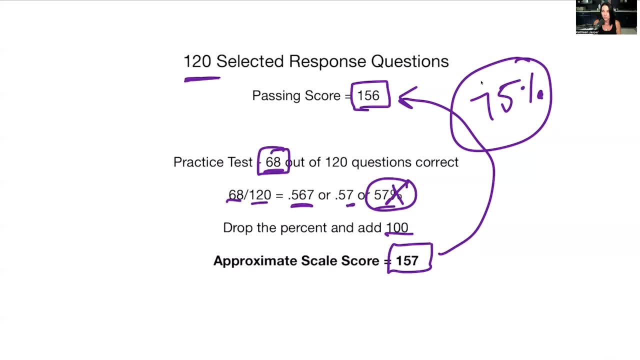 that sometimes that makes people feel better, But I always recommend to know that you have the readiness necessary to take the test and pass. I always shoot for a 75 on the practice test. That's my rule of thumb, But you can also use this formula. All right, let's talk about those. 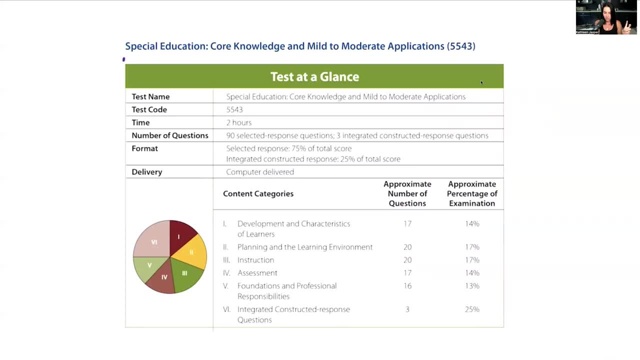 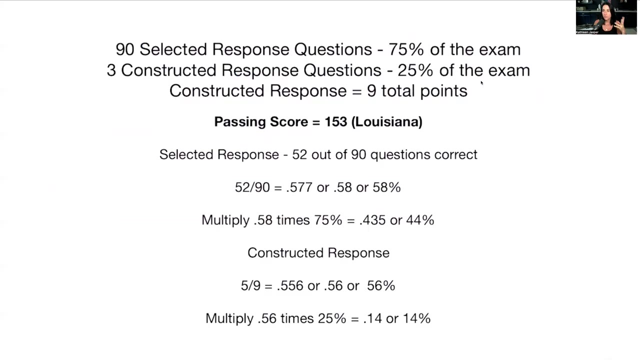 questions. So let's have a look at. this is the special education 5543. And this particular special education test has a constructed response portion. you can see that there are 90 selected response questions and three constructed response questions. Okay, so let me break this down to you. 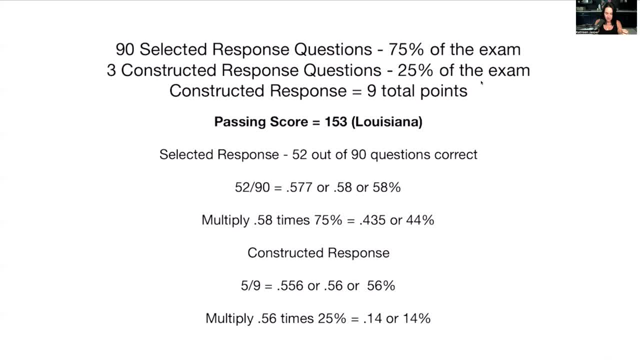 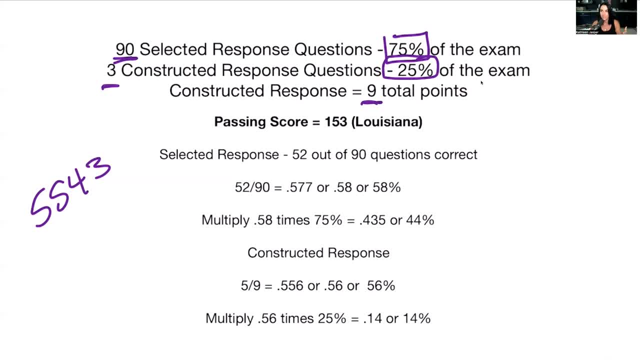 selected response section, you will see that the highest possible score you can get on each constructed response is a three. you can get a zero, a one, a two or three. So three times three is nine, which means there are nine total points up for grabs for the constructed response. So that's important when we need to know our total to figure out our percentage. Okay, So let's say on my practice test I got 52 out of 90 questions correct for the selected response. So my raw score is 52. 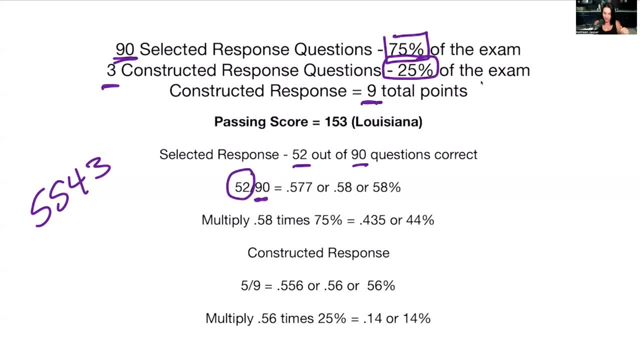 Well, I divide that by 90 to get my percentage, which, if I estimate here it's 58%, correct, All right, But I'm not done yet. That's only 75% of the exam, That's not the whole exam. So I need to multiply 0.58 or 58% by 75%, which gives me 0.435 or 44%. Now put that to the side. All right, Just put that number to the side. What we did here was we found our raw score. 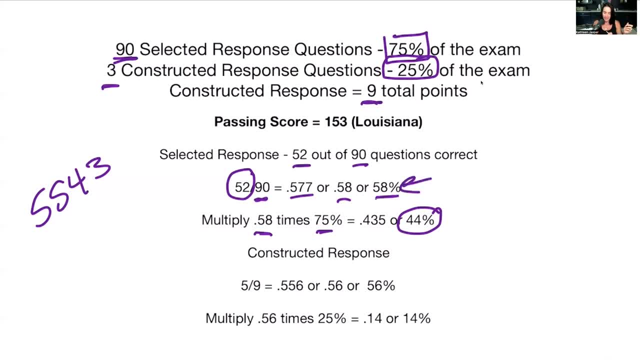 by the total. we got our percentage correct, which is here, And then we took that and multiplied it by the percentage that is of the overall score. All right, now for the constructed response. Let's say that I worked on my constructed response. I did my three responses And I decided to do a self assessment and look at the rubric and grade it myself, And I really recommend that you do that. you should write to the prompts and then grade it based on the rubric that's in the study companion, And so I have a 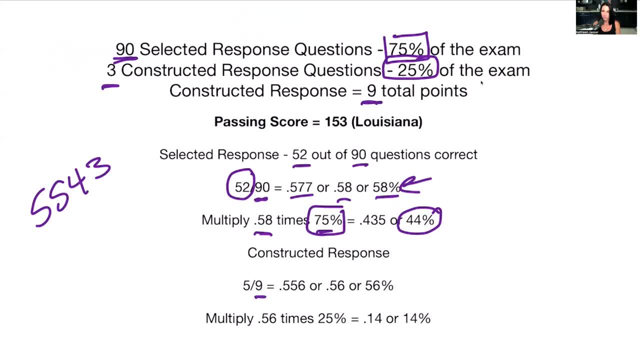 nine possible points, because three possible points for each one and there are three. So three times three is nine. And let's say that I gave myself a five, meaning I got a two on the first one, a one on the second one and a two on the last one, according to my self assessment. All right. So five divided by nine is 0.556 or 0.56 or 56%. All right, But that's not the whole test. It's only 25% of the exam, So I have to multiply 0.56. 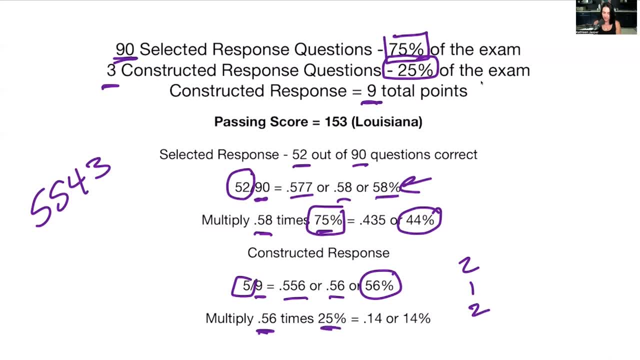 times 25% or 0.25.. And I get point one, four or 14%. Okay, so now I have the percentage that I got correct for 75% of my grade And I got the percentage I got correct for the additional. 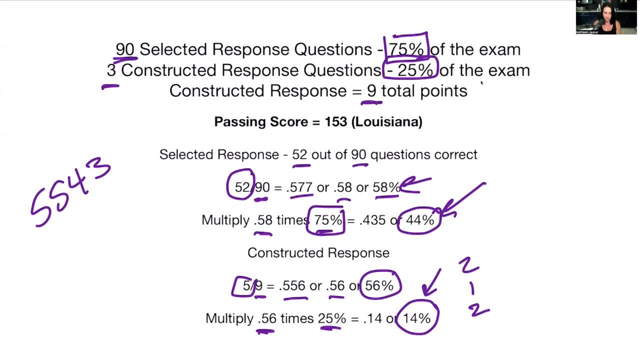 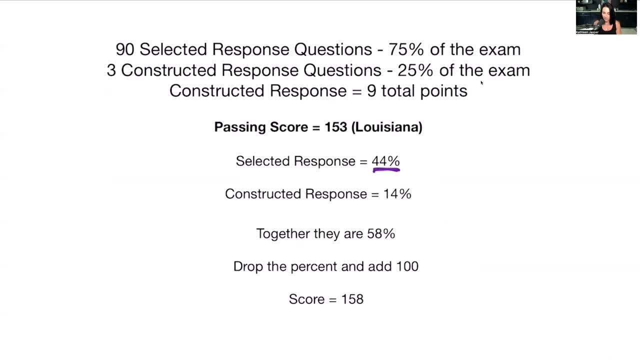 25% of my grade. These are the figures I'm going to use. Now what do I do next? Well, I take my selected response total percentage that I just calculated, And I take my constructed response total that I just calculated. I add them together and I get 58%. Now I can drop the percentage at a 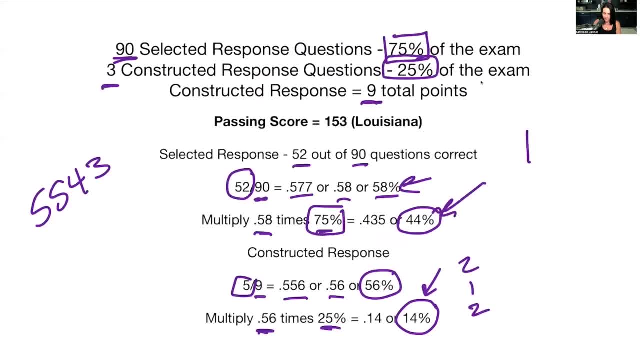 100. And I get a 158. Now, again, this 158 is pretty close to this 153.. In my opinion, it's too close, And so be careful, because, again, what we just did does not account for the weight of the questions. 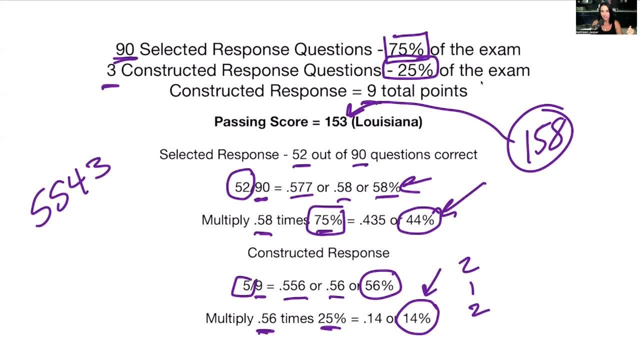 how complex they're going to be. any kind of curveballs you might get on the exam. So this is too too close. All right, I would say: if you did this and you got like a 165, something like that, you're in the safe zone. 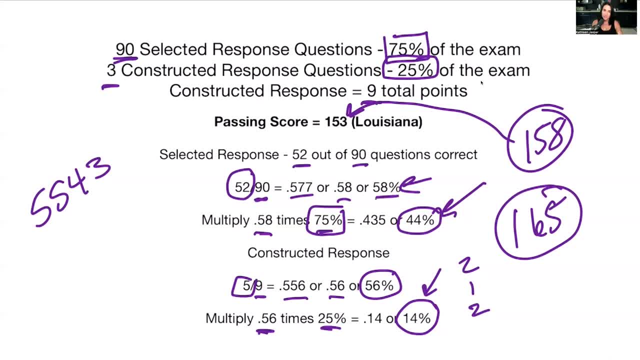 But still again, I always say 75% correct on the selected response And if you got 75% correct on this selected response, this low score on the constructed response would be okay, because that selected response would are the multiple choice, or selected response would push you up, All right. 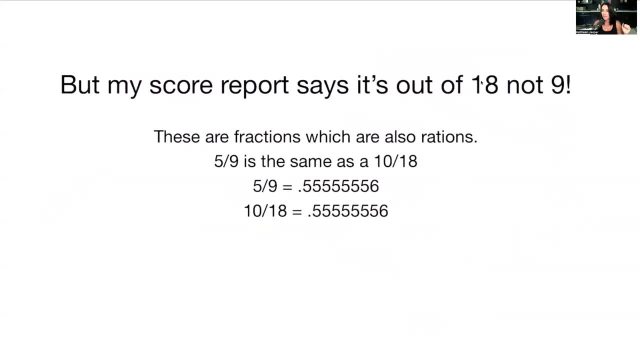 Now you might say: but my score report says it was out of 19 or out of 18, not nine. when I got my score report back, it said 18.. Well, yeah, these are ratios, they're fractions. Five out of nine is the same as 10 out of 18.. There. 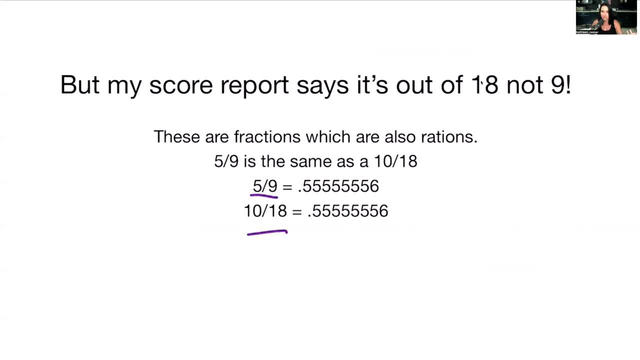 are two graders for your constructed response when it actually goes through the test right. So one grader gives you a set of scores and another grader gives you a set of scores, So it's going to be out of 18.. But regardless, it means the same thing: Five out of nine is the same as 10 out of. 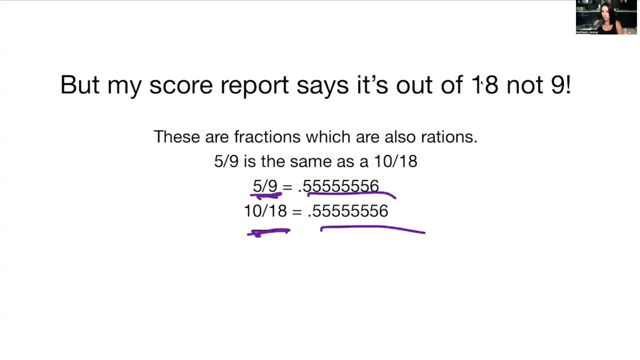 18,. you get the same measure there. So just remember that it's a. it's out of three, the multiples of three, 91824.. It doesn't matter, you're still going to get that same score because there are two graders at that. 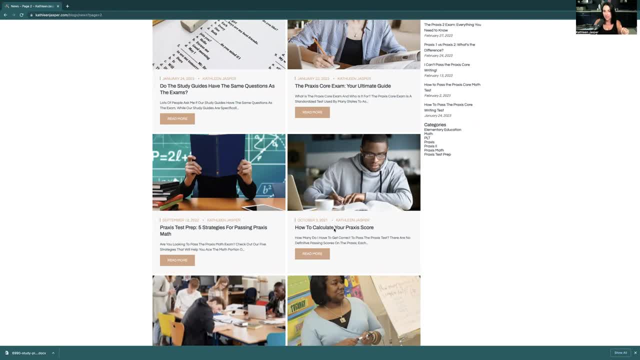 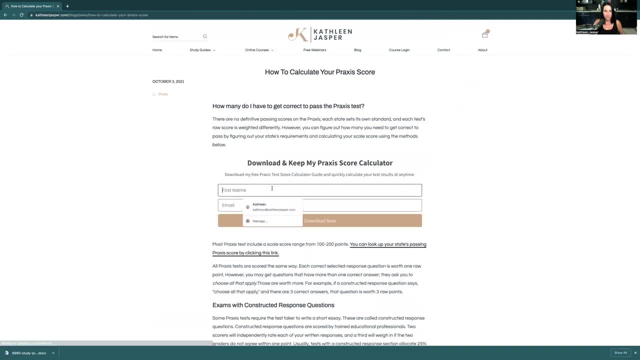 point. Now, I do have a score calculator. you can find it in this how to calculate your practice score blog And I'll hook that up in the comments below. But you can see that you can get the score calculator here And if I just enter my information and hit download now you get this little thing. 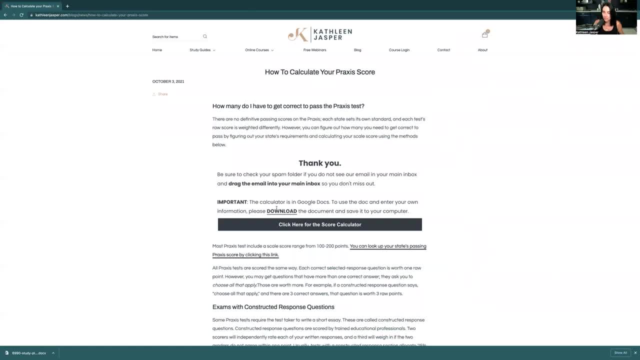 and you can hit now remember you have to download the document to use it. People, I get share requests from people. it says Hey, share the document. I'm not going to share the document with you because I don't want you to change the document. 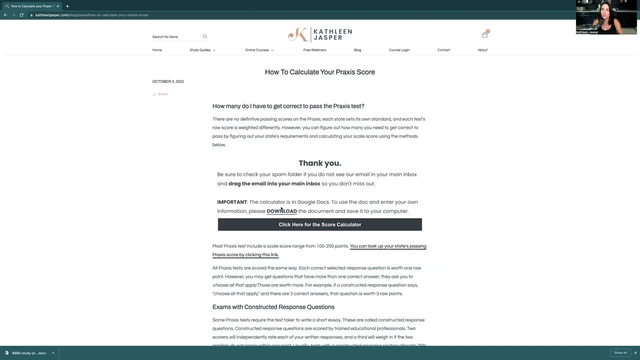 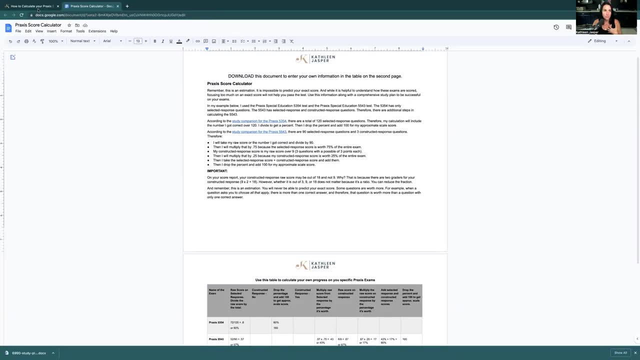 Because everybody's using it. you need to download it, save it to your computer And then you can use it. Let me show you what it looks like. This is what it looks like here. Obviously, it's on my drive, So it looks like this, but you need to go to file and download.